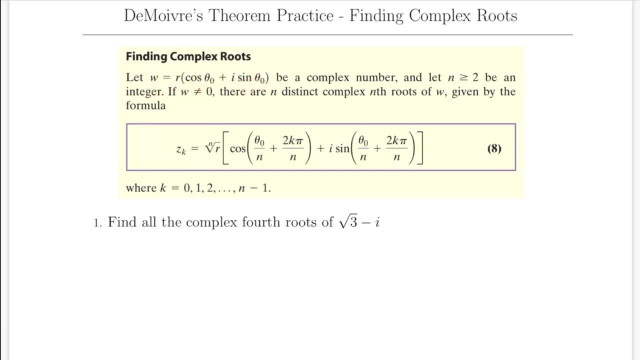 the number that we're going to find the roots of, and it's written polar form and that's where our R and our theta come from. in this formula is from that number in polar form. So that's often our first step that we have to do before we really even use this formula, because usually we're 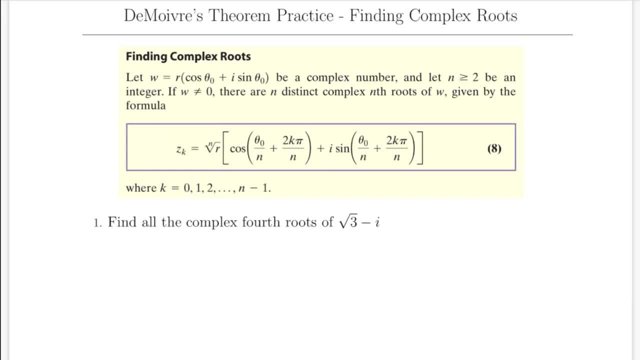 asked to find the complex roots of a number that isn't given In polar form, like this first example here. right? so first thing we're going to do is convert this to polar form. then we can start using this formula. Next couple things I want to point out are this: n. 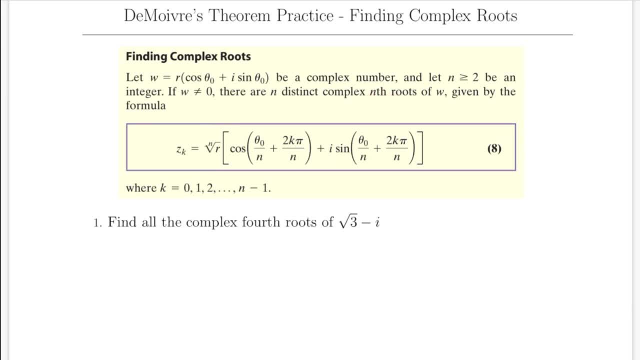 where does n come from? So n is the type of roots we are being asked to find. So in the case of this first example, we're being asked to find all the complex fourth roots of this number. So our n is going to be four right and there are going to be four distinct fourth roots of this number, and 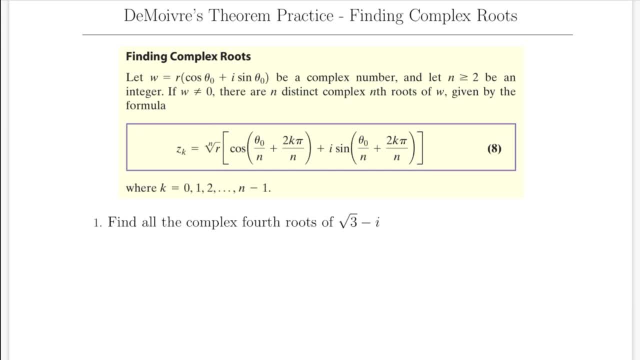 that's always true. So we're going to start by finding the complex roots of this number and then, if we're asked to find cube roots, then our n is going to be three and there are going to be three distinct roots. Those always line up, okay. So once we have R theta and we've identified n, we can plug. 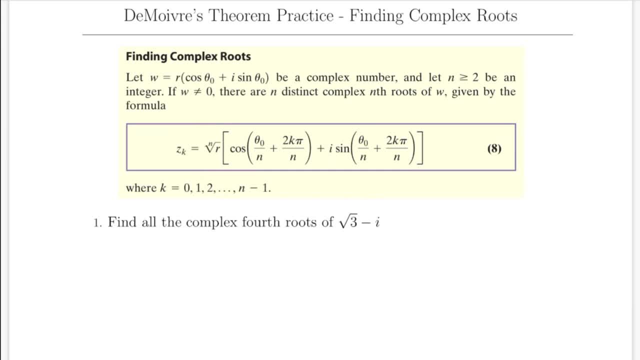 all that into this formula. and then the only thing that changes throughout using this formula is k right, and that's how we get each of our roots. We start with k equals zero. that gives us our first root, then we do one, that gives us our second root, and we continue until we find all of our roots. 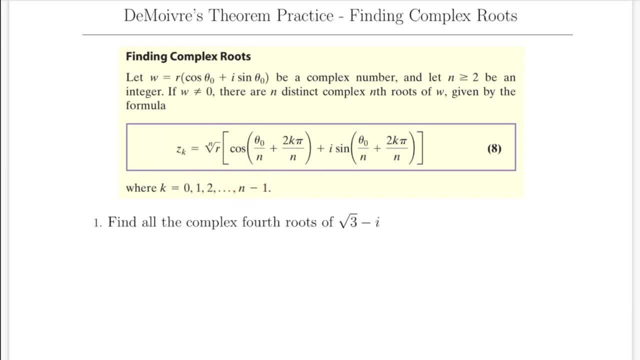 right, And that's why we always end up stopping one short of whatever our n is. and really it's just because we start this counting process at zero, right. So with my fourth roots, with this first example, I'm going to do zero, one, two and three, and those values for k are going to give me my four distinct 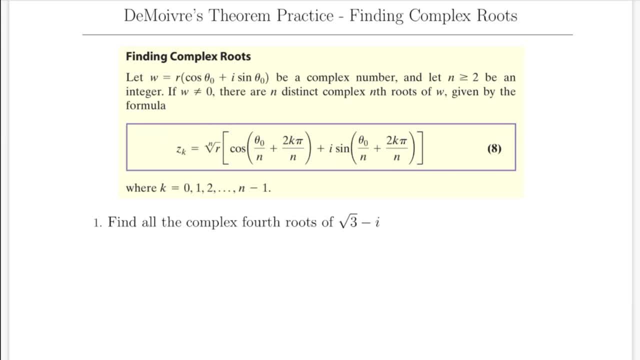 fourth roots. So hopefully that makes sense. This formula can be a little intimidating at first. it really just takes some practice getting used to it. Last thing I want to point out is there are different forms you can see this formula written in. Sometimes you'll see this combined into one single term. right, These common denominators, though this? 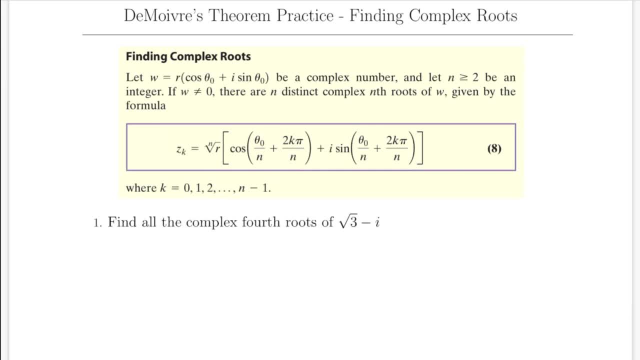 will be combined. Sometimes you'll see it written in degrees and actually that's the last thing I really want to point out before we jump into this first example- is that I actually prefer using degrees with these kind of problems, simply because we get to avoid dividing fractions and finding 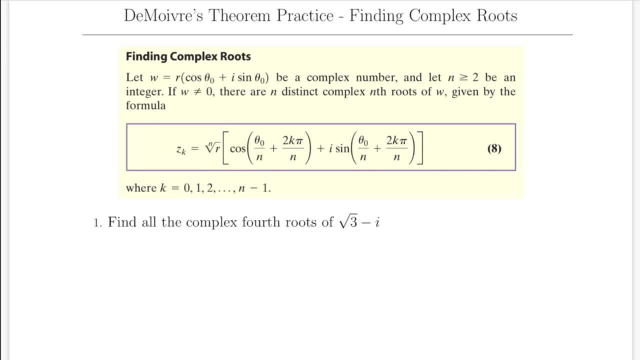 common denominators and that kind of stuff that comes along with using radians. So if you are going to use degrees, then really you just have to rewrite this and instead of using degrees, you just have to use your complex fourth roots. So let's get to that and I'm going to go ahead and write this case down. 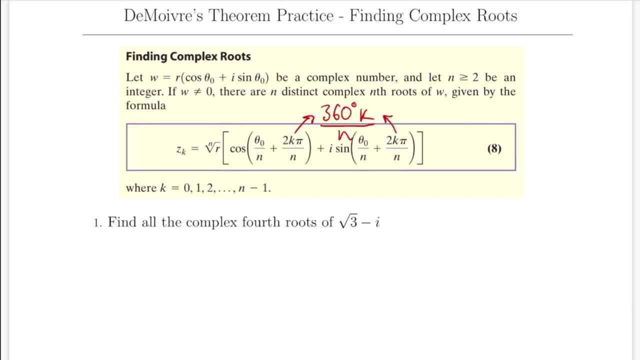 So this is at two pi. we have 360 degrees, so this will be 360 degrees k over n, and that will replace both of these terms, and then we can allow our theta to be in degrees, right? So that's what I'm going to use for this. 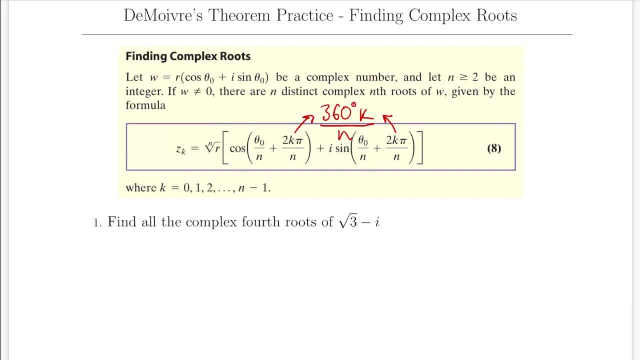 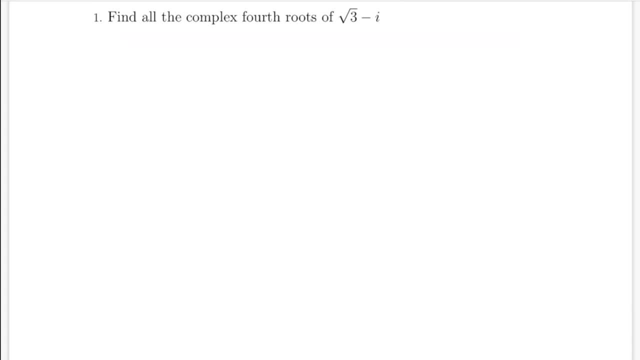 video. if you decide to use radians, that's totally fine. I just find degrees, at least in this context of using this formula, a little bit easier to work with. So let's go and jump into our first example, and the first thing we're going to do is convert to polar form. So what I like to do is plot this: 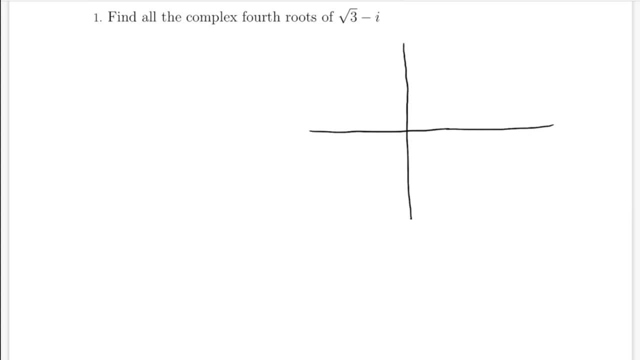 in the complex plane. and remember, this is my real axis, this is my imaginary axis, and the real part of this number is root three and the imaginary part is negative one. So I'm going to go root three along my real axis and then negative one along the imaginary axis, and this is going to be my 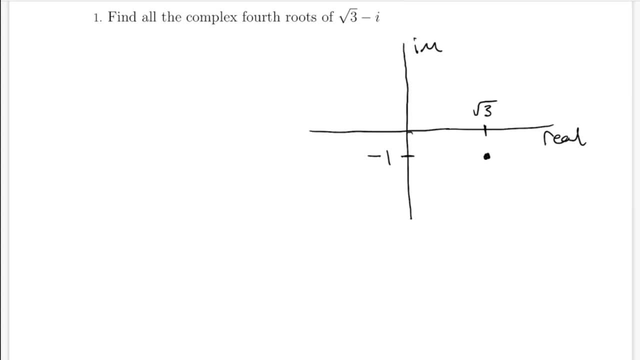 point right here, Okay, so remember that I'm trying to find r, so that's this distance here between the origin and the point, and I'm trying to find theta, so I'll draw my theta here in blue. that's this angle that wraps all the way around to this dotted line, right? so I need to find r. 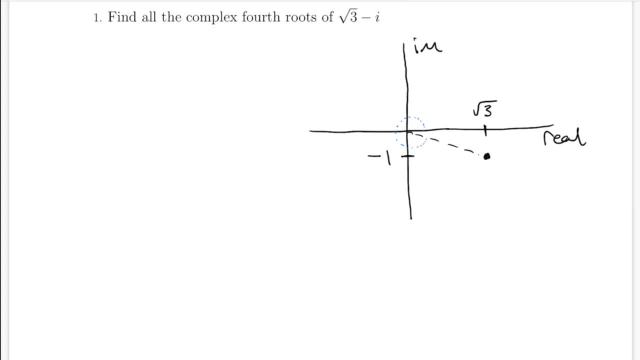 and theta. and I could start by finding r, because I can think of this as a triangle, as a right triangle, and then my r is the hypotenuse. so that means that r squared equals root, three squared root, three squared plus negative, one squared right. and, if you just remember, r squared equals x, squared equals y. 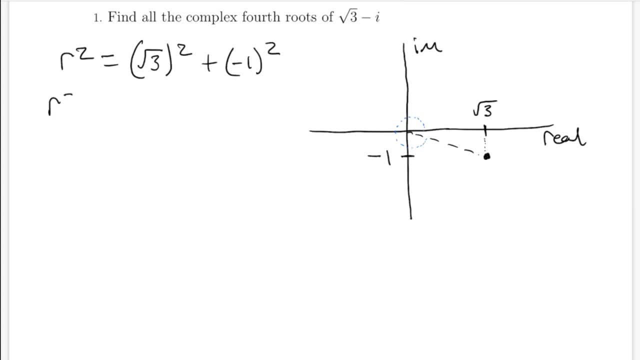 squared. that's exactly what. this is right. so r squared equals root three times root three, that's three. plus negative one times negative one, that's one. so my r squared equals four, and this means that r equals two. okay, so not too bad. r usually isn't too tough to find. now we just need to find. 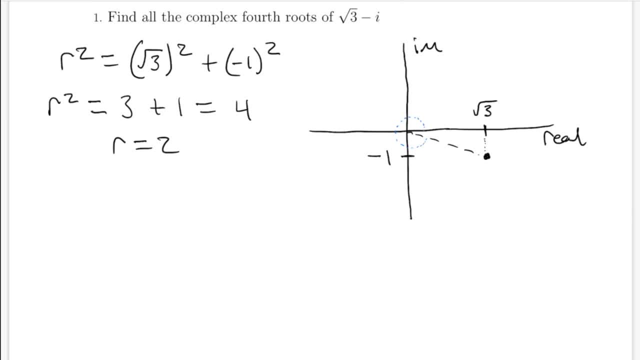 theta. so what I'm actually going to do is use tangent, Although you could use sine or cosine as well, now that we have r. but I'm going to say, whatever this angle is, the tangent of this angle equals y over x, right, or you can think of it as opposite. 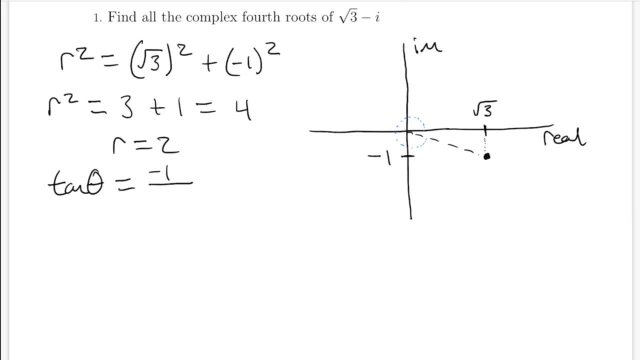 over adjacent, so negative one over root three. and if I rationalize this denominator by multiplying by root three over root three, it may look a little more familiar if you're thinking in terms of exact, because then what I get is: I'm looking for an angle where the tangent of that angle is equal to. 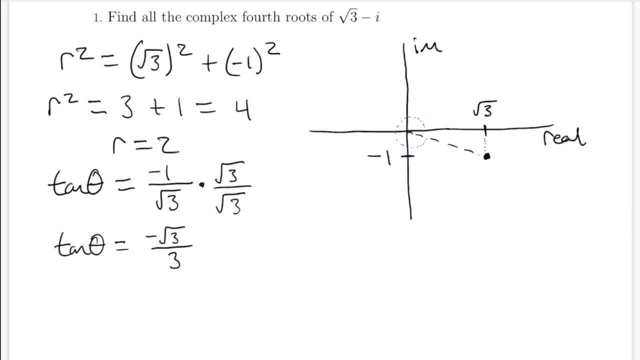 negative root three over three. okay, since it's a negative, I know it's either going to be in the second or fourth quadrant, but obviously we're in the fourth quadrant, so I'm looking for the angle in the fourth quadrant and I know that for these kind of root three over three values our reference. 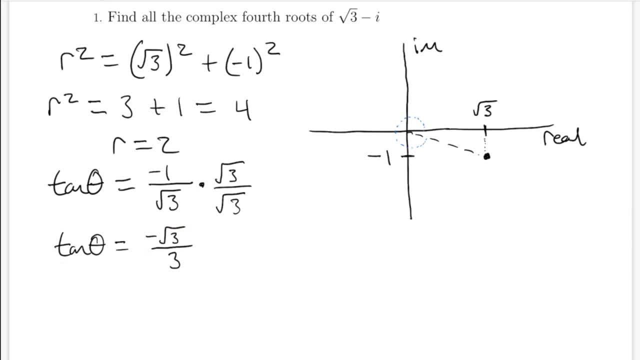 angle is always 30 degrees when it comes to using tangent. so that means I know that this angle, here our reference angle, is 30 degrees. so that means that, wrapping all the way around I'm going to be. I'm stopping 30 degrees short of a full rotation. so then, my theta in this case is actually going to be: 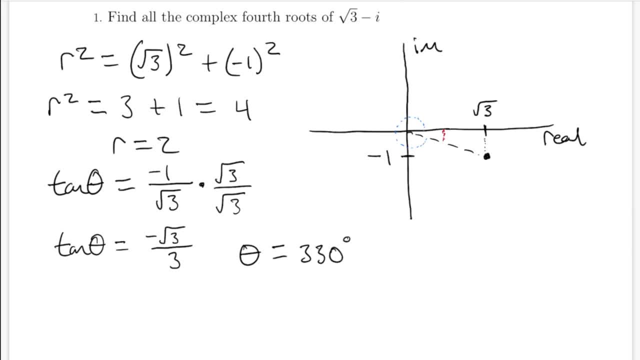 330 degrees. and now we found r and theta, so you could take theta equal to negative 30 degrees, and that would technically work. however, when we use this formula, I like to have my angle as a positive angle measure between zero and 360, right, so I'm taking this one. so, now that we have r and theta, 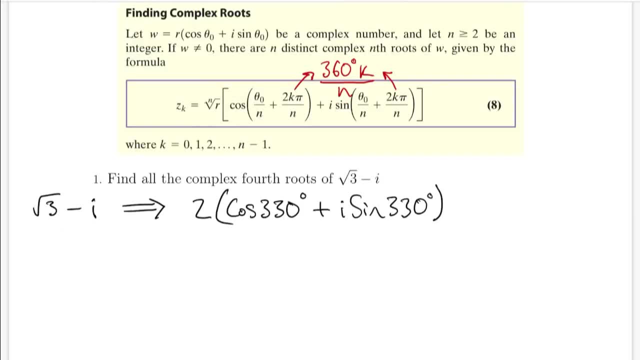 let's see if we can rewrite this number in polar form. all right, so I've taken this number, I've converted it to complex polar form and now I'm ready to start using this formula to start finding the fourth roots of this number. so I'm going to start by 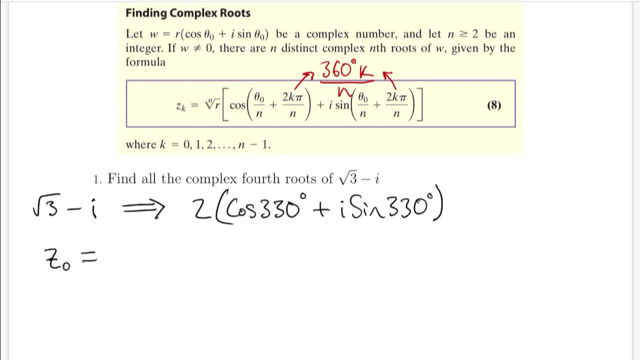 finding my first root, and remember that's when k equals zero, and what I'm going to take is the nth root of r. so my r in this case is two, my n is four, so I have the fourth root of two and I'm just going to leave it like that, because there's no nice way to simplify that without. 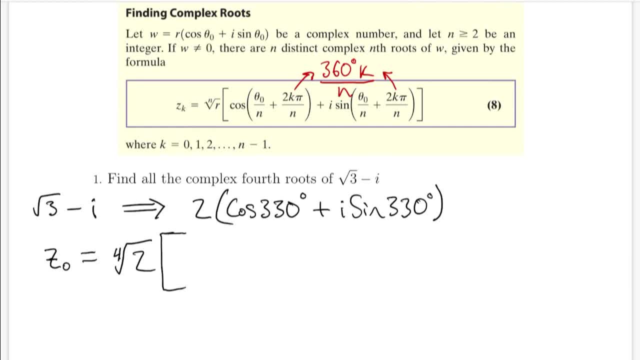 having to put it in a calculator around, and I don't want to do that. so I'm going to take this and I'm going to do that. so then what I have in here is the cosine of theta over n. remember, my n is four and my theta is 330 degrees. so 330 divided by four, that should give me 82.5 degrees, okay, plus. 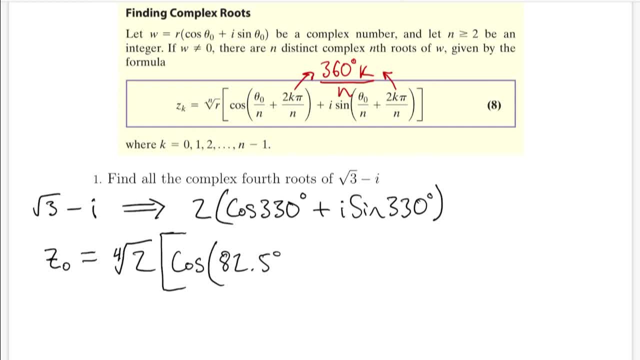 360 degrees k over n. well, my k is zero, so it doesn't really matter what n is. when k is zero, that term is always going to disappear, so I end up adding zero here, so I can really just forget about that term. and that's always going to be true. when we find 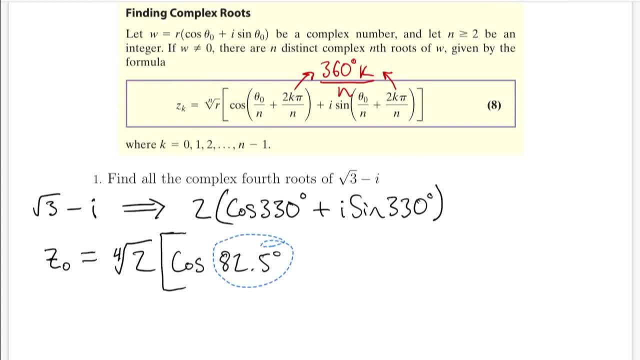 our first root when k is zero is: we can just forget about that. so here we just have the cosine of 82.5. and another thing I want to point out is that the argument for cosine and sine right- the stuff that's in the parentheses- is the same. so once I find this for cosine, I can just write. 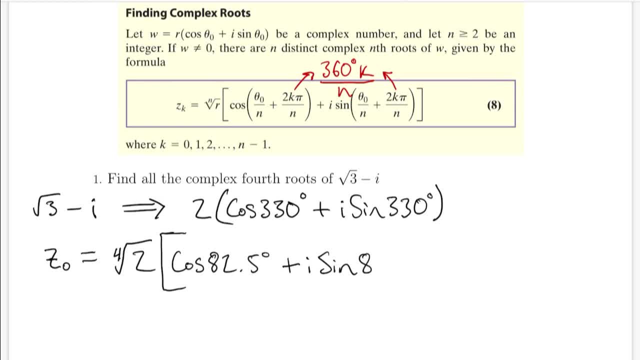 it down for sine. there's no sense in trying to work it out again, because I've already found what I wanted to find, right, so I can just copy the rest down and bam, there we go. we have our first root, so let's see if we can. 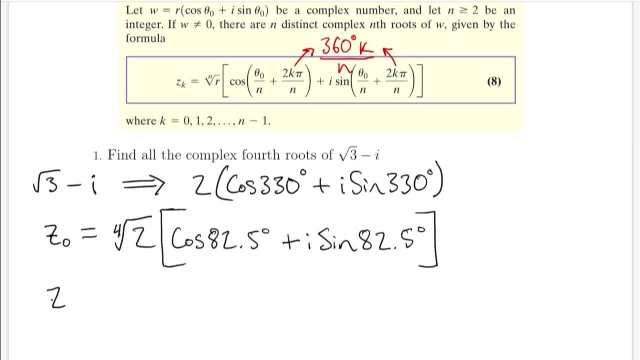 find our second one. so that's when k is equal to one and the nth root of r. that's always there, right? it doesn't matter what k is, so I can just copy down fourth root of two, and then I can write out the cosine of and remember theta over n. that doesn't change either. 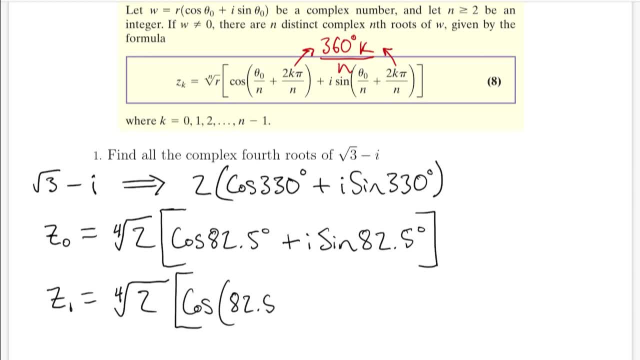 so I can write out 82.5 degrees and all I have to think about is: what am I? what am I adding now? right, so I'm adding 360 degrees times one over n. n is four in this case, right? so 360 divided by four. 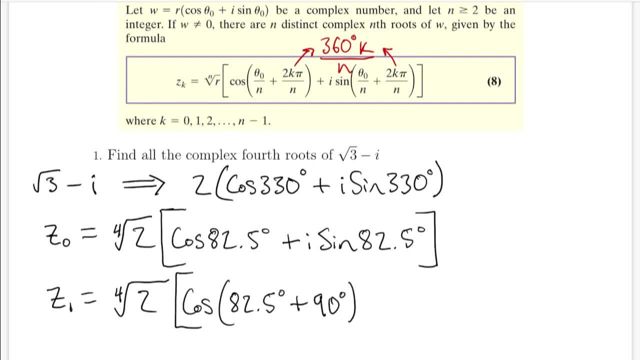 that's 90 degrees. so I'm taking 82.5 and adding 90 degrees, and that's going to give me my argument here. so when I add those together I get 172.5 degrees. so I'm just going to go ahead and replace. 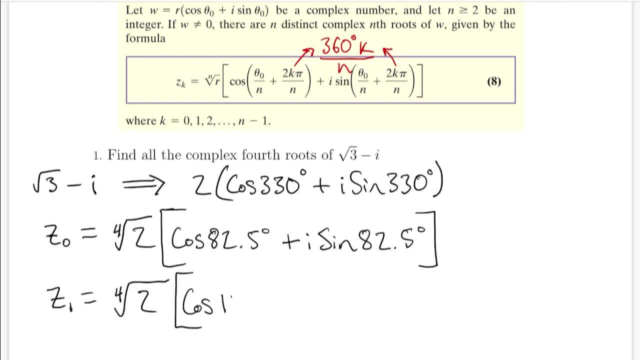 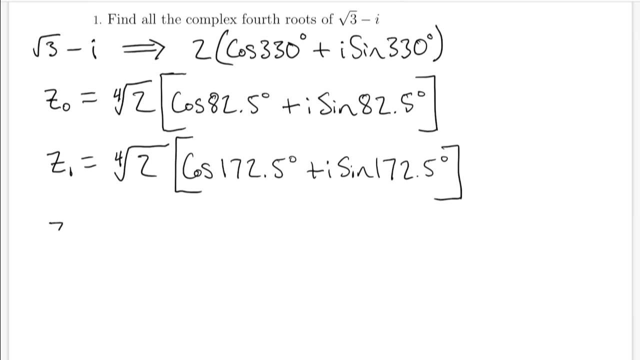 this with 172.5 degrees and remember, once I find the angle that's in the cosine I can just copy it down. first sign: those are always the same. so plus i sine of 172.5 degrees and we found our second root. we just have two more to go, so I'm going to scroll down. so the next root is: 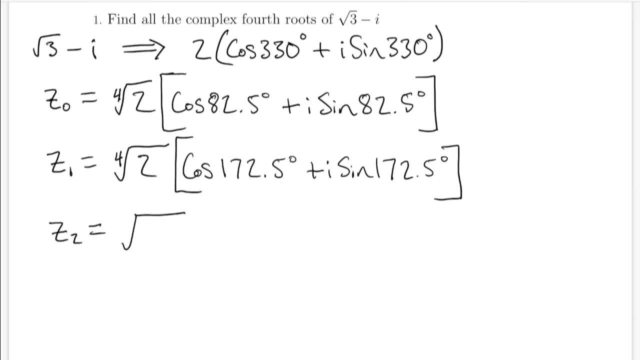 when k is equal to two. and again, we can always just copy it down: what's in front here? fourth root of two times cosine of: remember. this is theta over n. this is the over n. that's always going to be 82.5 degrees. We just have to figure out. what are we adding? 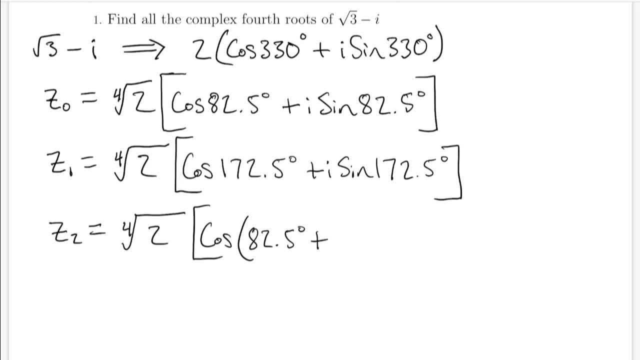 now that k is equal to 2.. Well, we have 360 times 2, that's 720, divided by 4, that's going to give us 180 degrees. So when we take 82.5 degrees and add 180 degrees, we should: 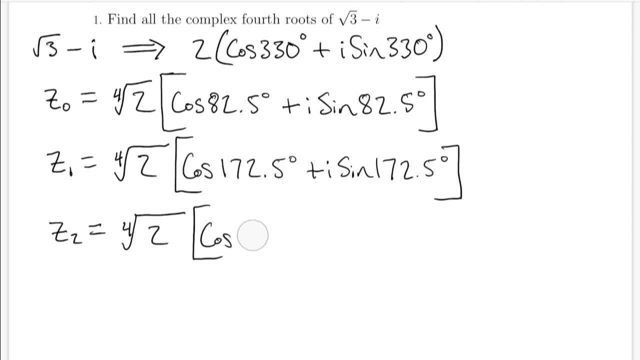 get 262.5 degrees. So I'm going to go ahead and replace this with 262.5.. And again, I can copy this down for the sine part as well. plus i sine 262.5.. And now we just have one. 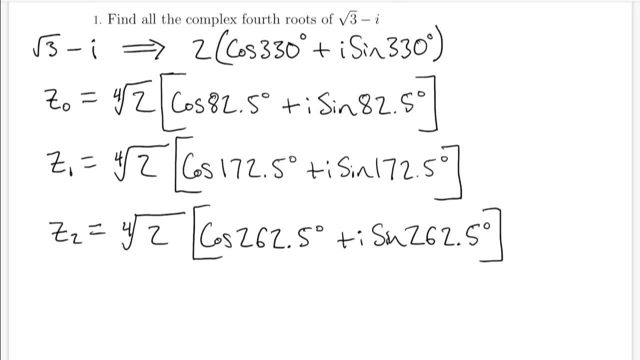 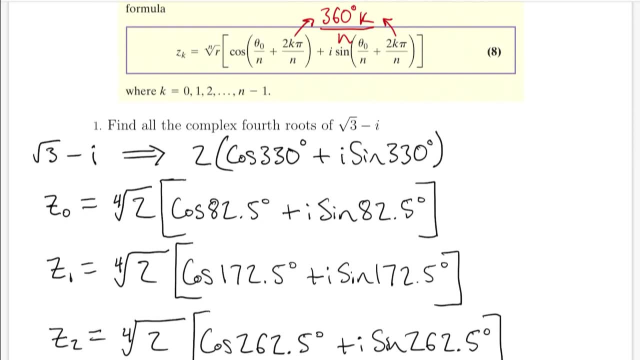 left, And maybe you know that there is a pattern here and I'm actually going to point that out right now. And one way to see it is that each time we increase k by 1, we can think of the same thing. We can think of the same thing as the same thing. So we can think: 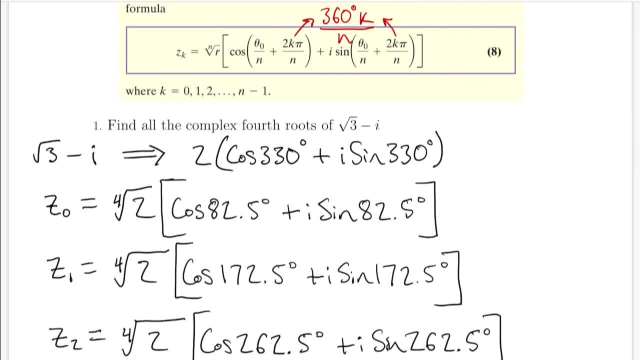 of the same thing as the same thing. So we can think of the same thing as the same thing. We can think of this multiplication as repeated addition, right? In other words, look at the difference between the angle in my first root and in my second root: 90 degrees. right Now look at. 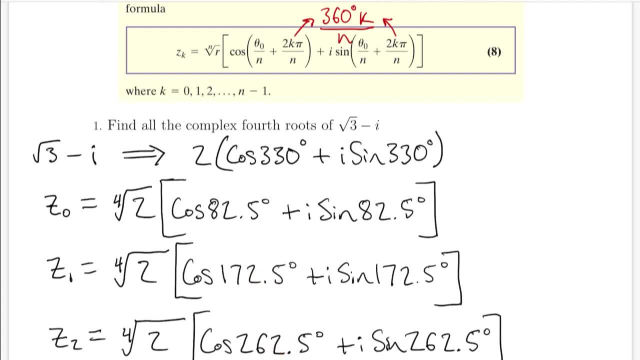 the difference between the angle in my second root and my third root: 90 degrees. That's always going to be consistent, right? Because each time I increase k by 1, I'm basically just adding another 360 degrees over n, right? In other words, if k is 2, then really what I'm doing is 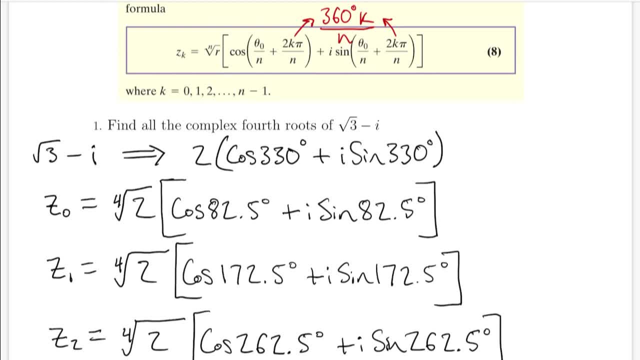 multiplying something by 2, which is like adding it twice, Multiplication can be thought of as repeated addition. So in other words, I'm repeatedly adding this 360 degrees over n k times to this angle right. So if we follow this pattern, what we can notice is 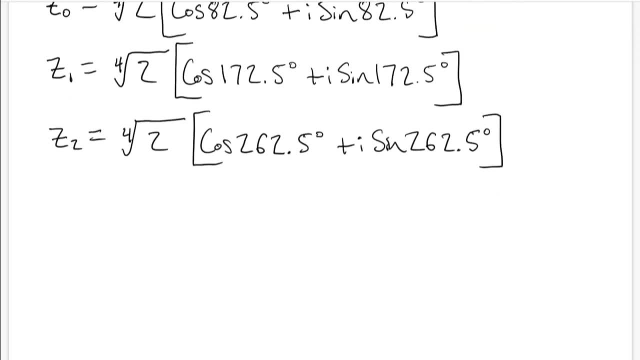 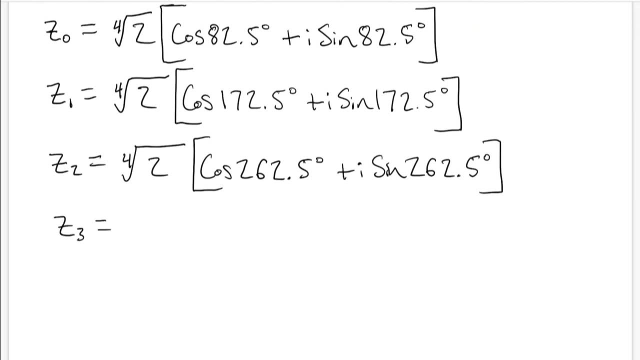 that, oh, from each previous root to each next root, we're just taking the angle and adding 90. And that's actually a nice little shortcut. And if you knew that already, then maybe you're frustrated that I worked all of these out by hand the way I did, But it's. 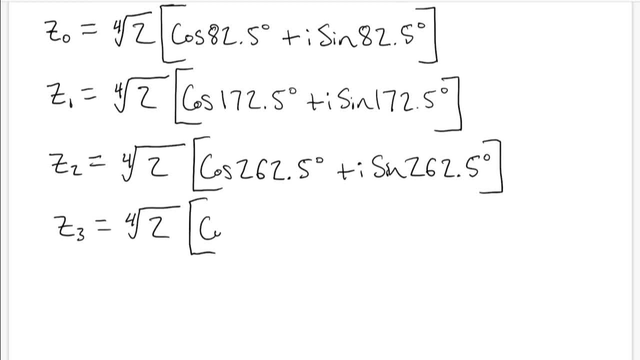 since a lot of people watching this video are probably just learning about this formula, I wanted to show me working it all out. But in the future, in the next example, I will use this pattern where we notice that add 90,, add 90,, add 90. So this is going to give me. 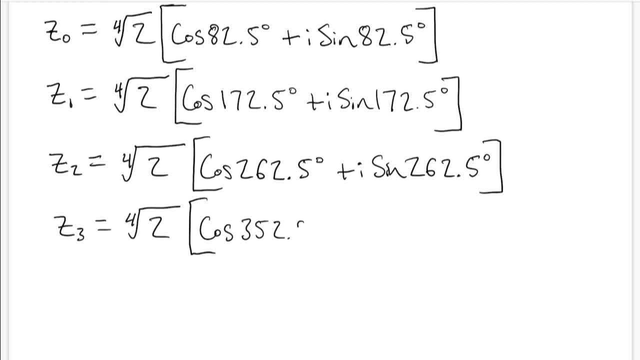 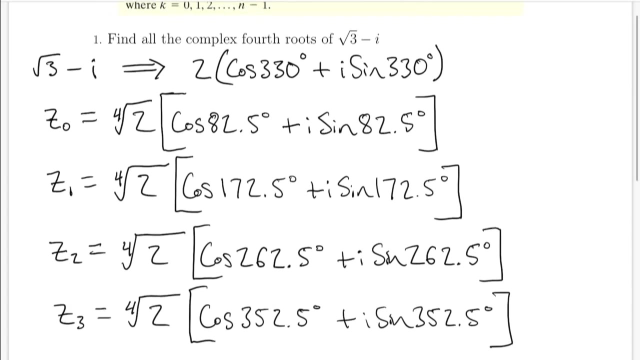 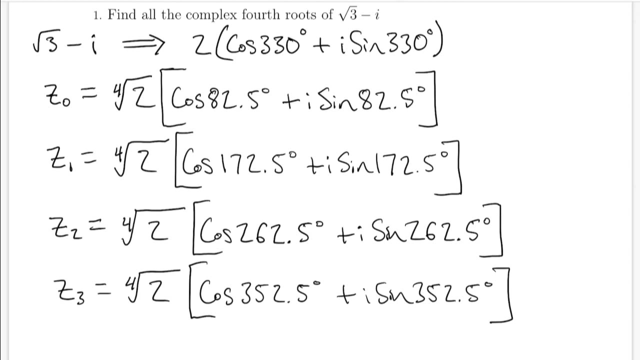 352.5 degrees plus i sine 352.5 degrees. And those are all four complex fourth roots of root 3 minus i. We could convert these to rectangular form If it was asked in the question. we would just have to use a calculator. I'm going to leave. 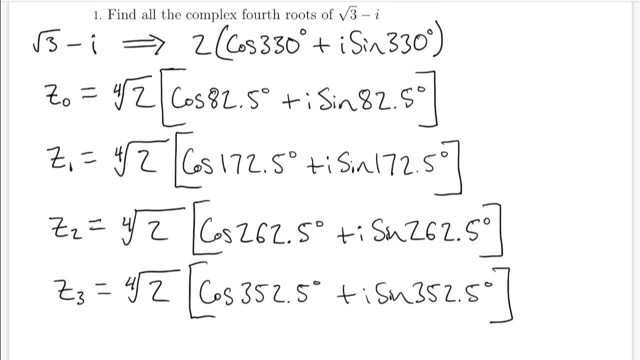 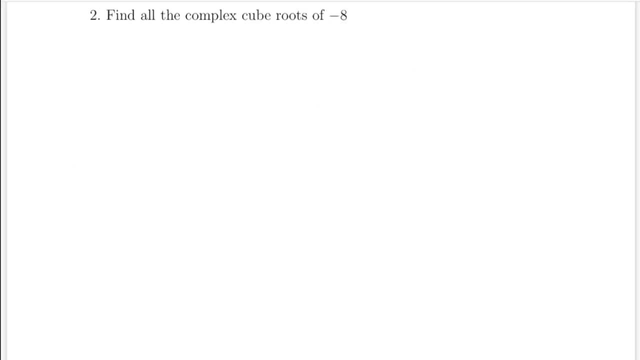 them like this. Usually it's okay to leave them like this, But hopefully that example helped. We're going to do one more and then we'll finish up the video there. All right, so now we're going to find all the complex cube roots of negative 8.. And at this point, 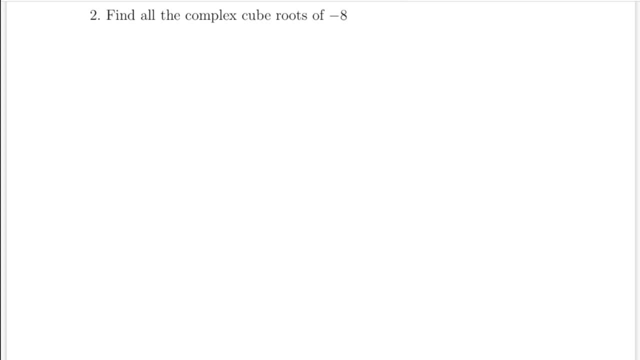 I actually encourage you to pause the video and try this on your own. Then press play to compare your work with my work. But we're going to go ahead and start by converting this to polar form. We need it to be in polar form in order to use our formula And what I see a lot of students get confused about. 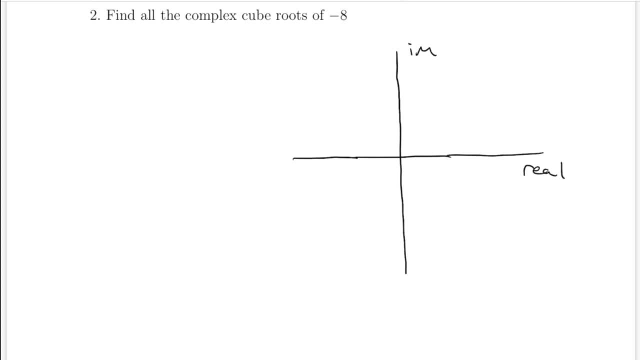 with these kind of examples is: where is the imaginary part of this number And what I like to write this as is negative 8 plus 0i, and that often clears it up. So my imaginary part is actually 0, right, So I'm going at negative 8 along the real axis and then 0. 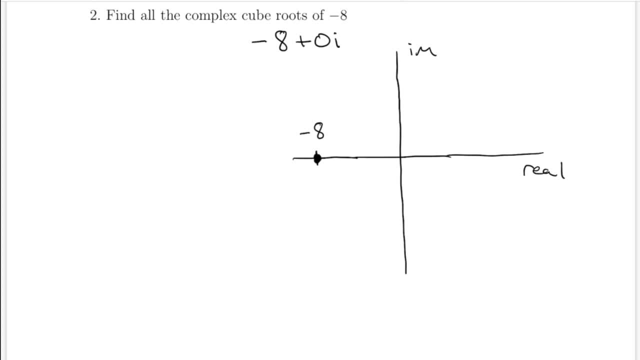 on the imaginary axis, So my point is actually here on the real axis. And this is a great example of why I like to plot these in the complex plane, because we can actually visually see what our r and theta is. Remember, our r is the distance from the origin to that. 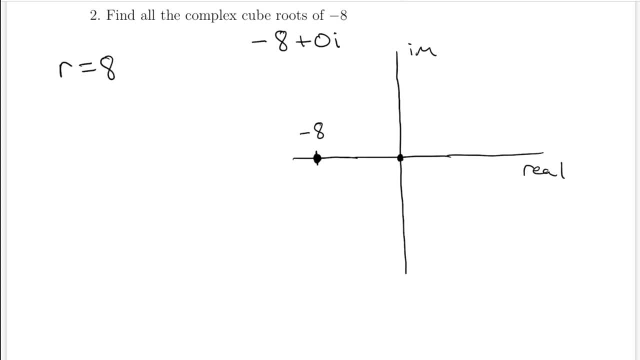 point, which is clearly 8, right. This distance is clearly 8 here, And our theta is this angle that takes us out to this line that extends out to negative 8, right. So in this case our theta is actually 180 degrees, So it's pretty clear to see both. 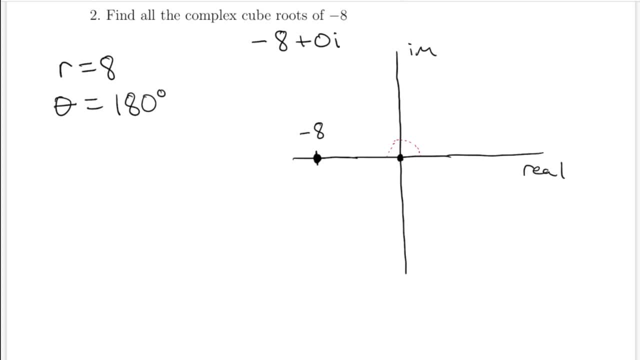 of these, and we didn't even have to really do anything other than just look at the point we plotted in the complex plane. So that's why I like to do this. Now let's see if we can write negative 8 in polar form. So negative 8 converting to polar form. So we have r. 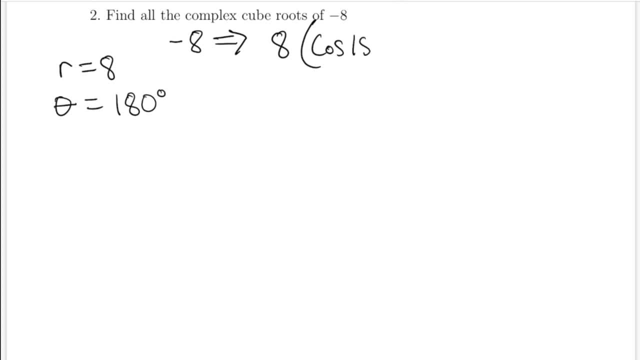 and then we have the cosine of 180 degrees plus i sine. So negative 8 is going to be negative 1 over 180.. So now this is the number in polar form that we're going to use to find our roots. So first, when k is 0, what do we have? Well, 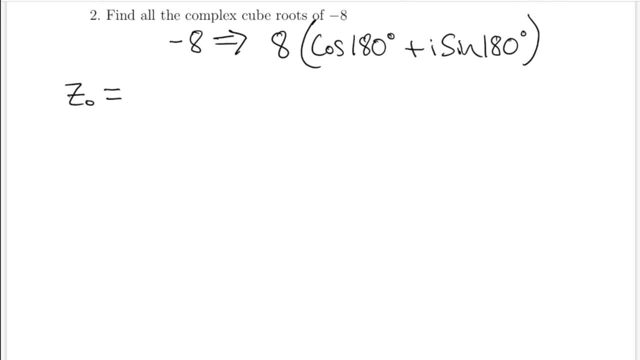 remember, our n is 3.. We're finding cube roots, So we're going to have 3 distinct cube roots. Since our n is 3, what's going to be out here is the cube root of 8, which we can actually 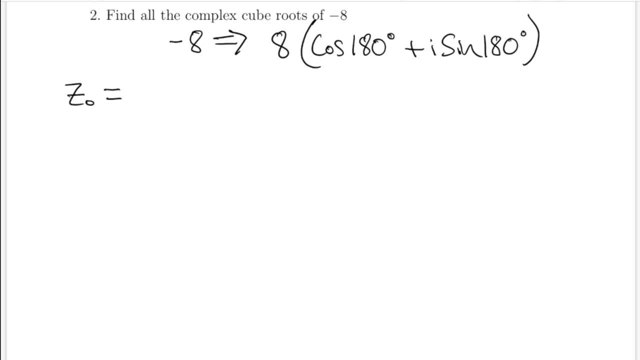 nicely simplify, because that's just 2, right 2 cubed is 8. So we can replace that with 2.. And then what we have here is the cosine of 180 over n, So 180 over 3, which gives us: 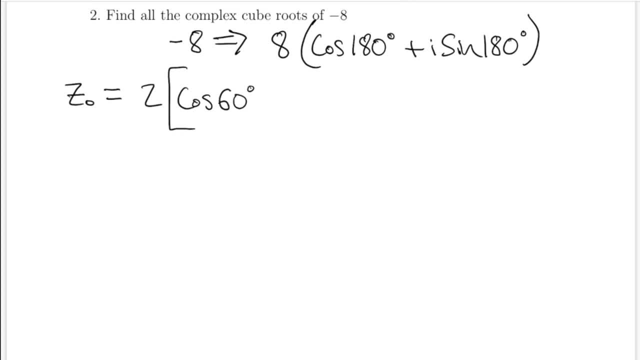 60 degrees, And remember, that term that we're adding has k in it and since k is 0, that always disappears when we find our first root. So this is the angle in our first root And in this example I'm actually going to employ the shortcut that I mentioned in the last. 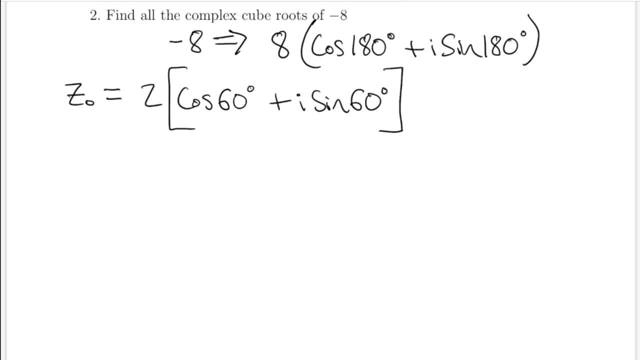 example, that pattern that we noticed. So that principe would be: if you make the limite to 2, what would be the first time you looked at Ge drama? If you take a look at the cytographic example, it says: if you 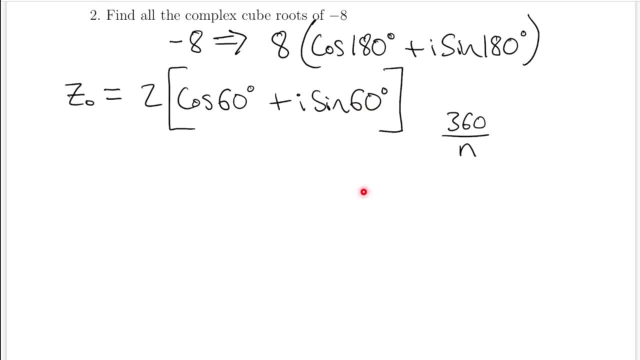 want to paused the segunda sets or the integral of 0,. you want to basically just take a look at theרת of 9, and you increase it. So the first time we had our 39, and the second time we made our grille of 60. And theirting set. we wanted to notice because we could. 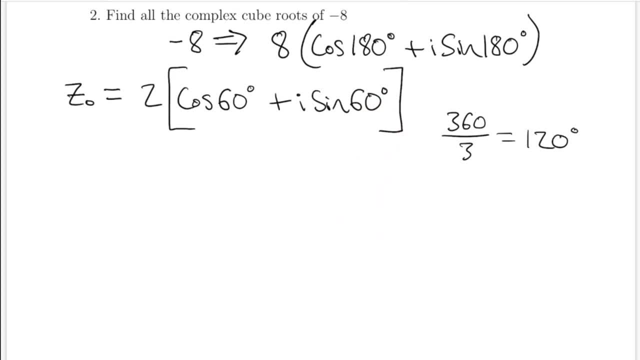 to get to each angle in our next root, and the reason why this is again is because we have a k attached to here in our formula. so when k is 1, we're adding 120 degrees to 60, and when k is 2, we're adding 120 plus 120. that's why i was mentioning that repeated addition. if that. 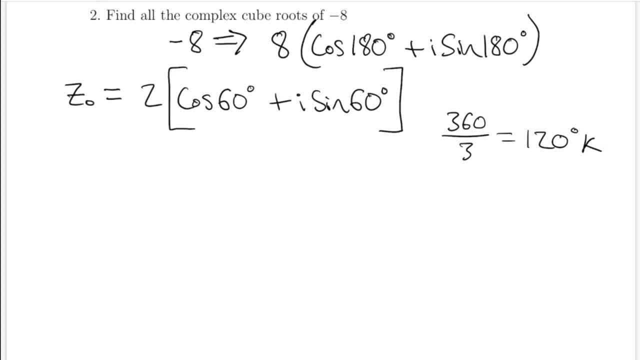 didn't make sense. maybe this is a little clearer. so when k is 2, we're adding 120 twice to 60, and that's why we can just add 120 to each previous angle to get to each next angle. hopefully that makes sense. let's go ahead and employ this little pattern. you'll see it makes this process a lot. 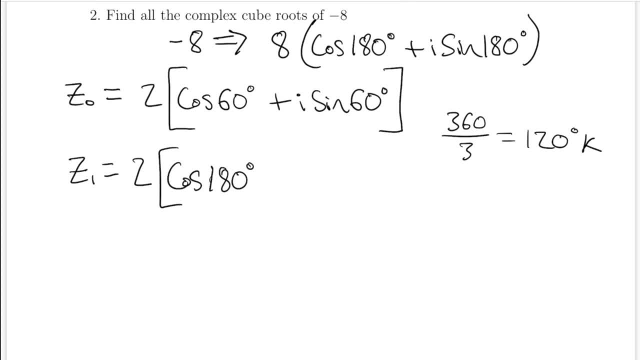 quicker, because now i can just write this as 180 degrees, because that's 60 plus 120, and then my next root is going to have 300 degrees in the argument and what's out in front here always stays the same. so i don't need to change this at all. right, because that's just the nth root of r, which never changes. 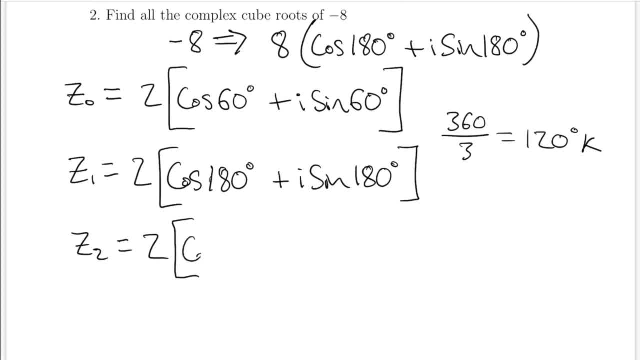 the only thing that changes is my angle, so i can just write this as 180 plus 120, so 300 degrees, and it saves you a little time, and so this is how i usually do. it is off to the side. i just write out whatever my 360 over n is, and it really just depends on what kind of root you're. 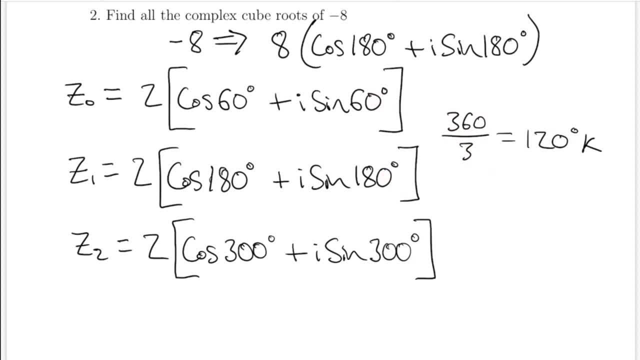 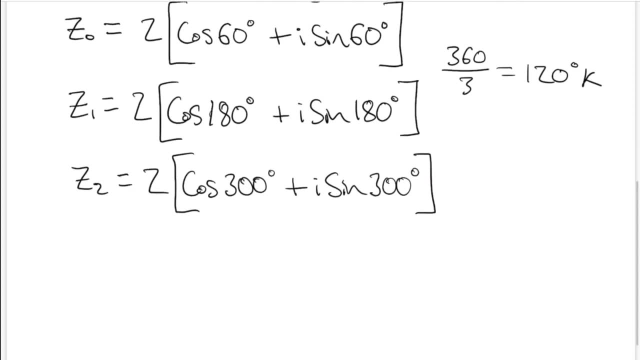 finding, and then that's the angle that i add each time to get to each next root. so these are three distinct complex cube roots of negative eight, and what what i'm actually going to do for this example is convert each of these to rectangular form, just so we can see what that looks like. 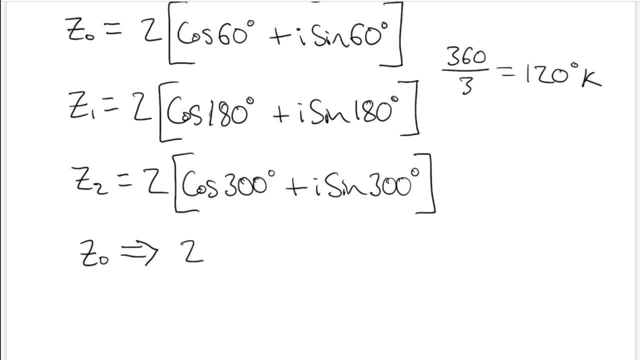 and just because it's pretty easy. we actually don't need a calculator because these are all exact values that hopefully we know. cosine of 60 is one half, sine of 60 is root 3 over 2, and then i'm going to convert each of these to rectangular form. and just because it's pretty, 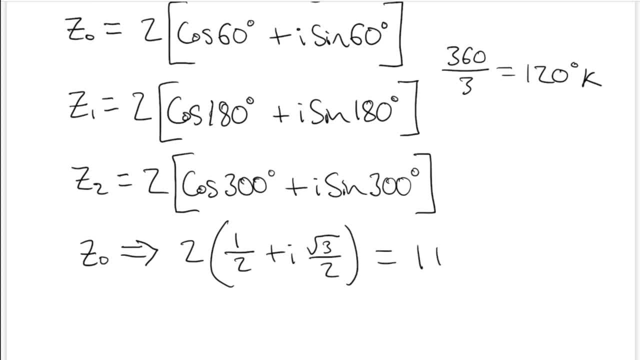 easy. we actually don't need a calculator because these are all exact values that hopefully we know my twos cancel out nicely. so one of my roots is one plus root 3i. and now, if you remember, when you took algebra, we always have these complex conjugate pairs as our roots. so think about that. 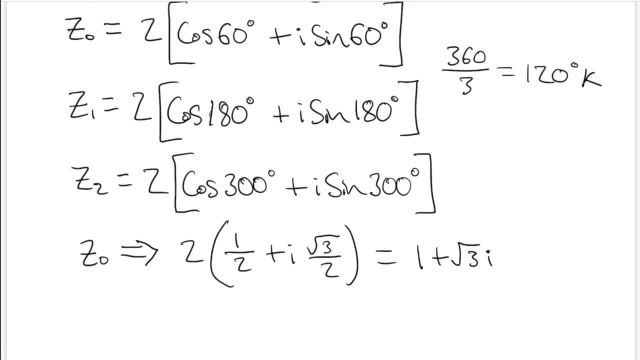 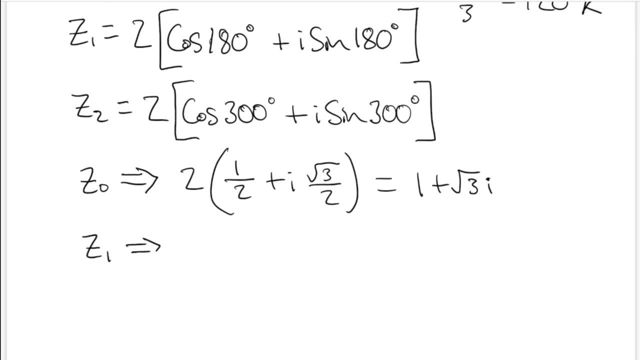 one of our roots should turn out to be one minus root 3i. right, we can kind of look ahead at that. so let's see, if we convert our z1 to rectangular form, we get two times. let's see cosine of 180. that's negative one. 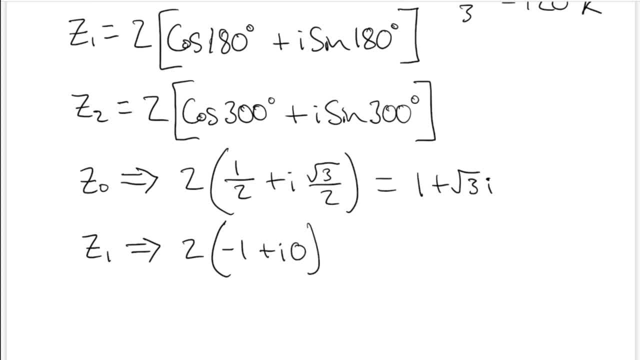 plus i sine of 180, that's zero. so my i term actually disappears there and i'm just left with negative two. let me write that two a little better, but that should make sense, because, think about it, negative two cubed is negative eight, and that's really what we're being asked to find are. 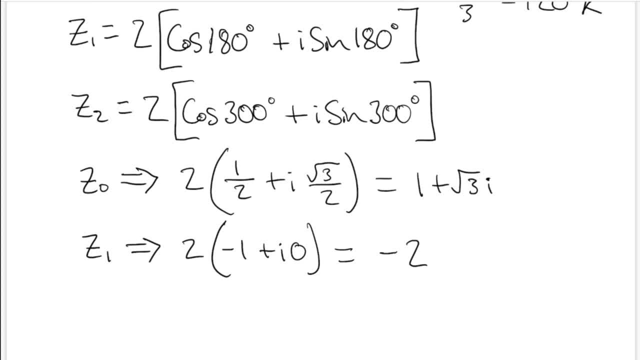 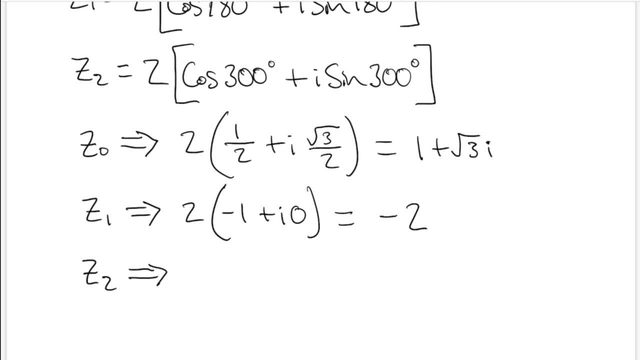 all the numbers that we can cube to get negative eight right. so that should make sense as well. and then we're expecting this one to be that complex conjugate pair, so we're expecting this to be one minus root 3i. but let's double check for sure. cosine of 300, that is one half plus i. sine of 300, that's negative. 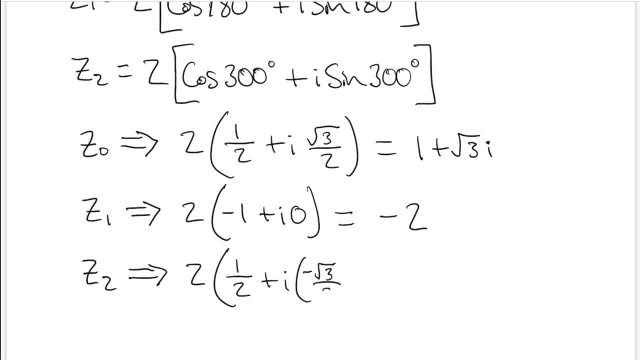 root 3 over 2, so i'll just write it here in parentheses. but once we simplify this, this ends up being 1 minus root 3i, which is what we suspected it would be, and then we have our three roots, now in rectangular form, so this may not be required, but i think it's cool to kind of relate this to. 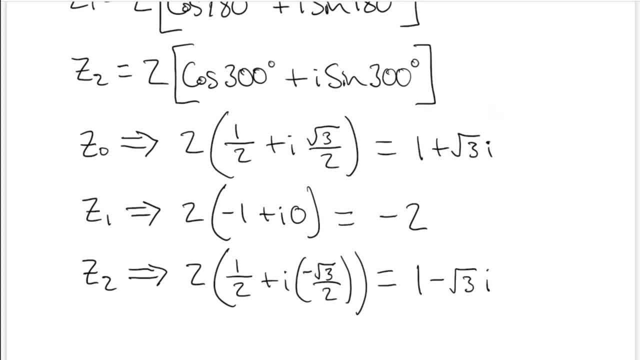 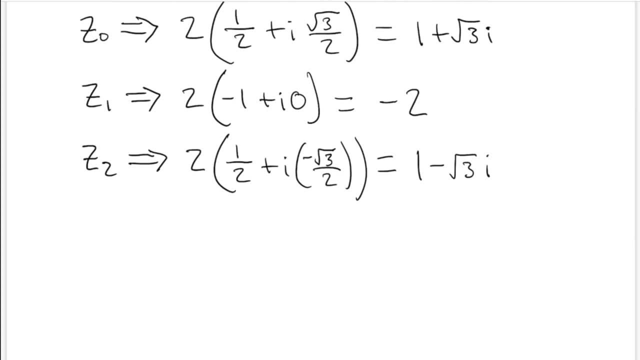 stuff that we've done previously in algebra, and that's kind of one. last thing i want to point out is that we can actually, when dealing with numbers like negative 8, negative 27, negative 1, and we're finding the roots of these, we can actually do this without using de mar's theorem. right, we could have. 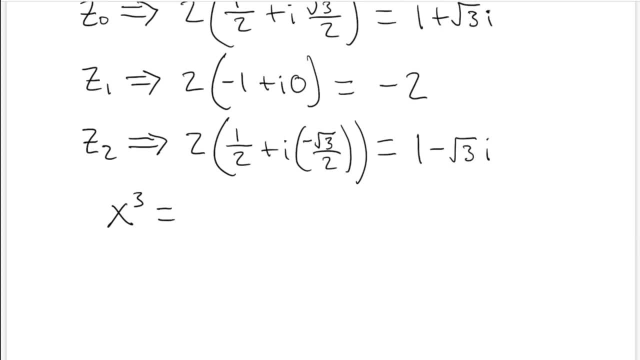 just wrote out: well, what number can i cube to get negative 8, because again, that's what we're asking to find here, right? and then what we could have done is: solved this equation. this is actually a sum of cubes, right? so if we factor this, we have x plus 2. 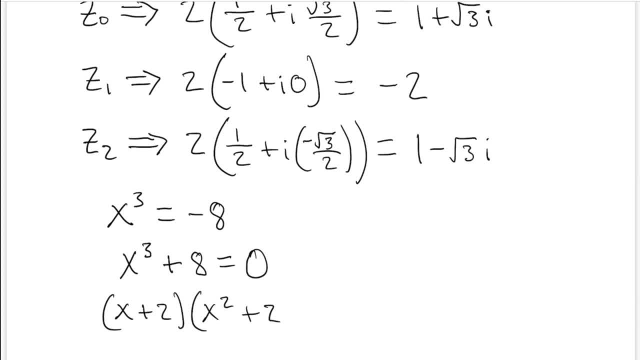 times x squared plus 2x, let's see same opposite, always positive. so this is actually a minus plus 4 equals zero. okay, when we set this part equal to zero, we get our negative two root. and when we set this trinomial equal to zero and solve, we get that complex conjugate pair right. 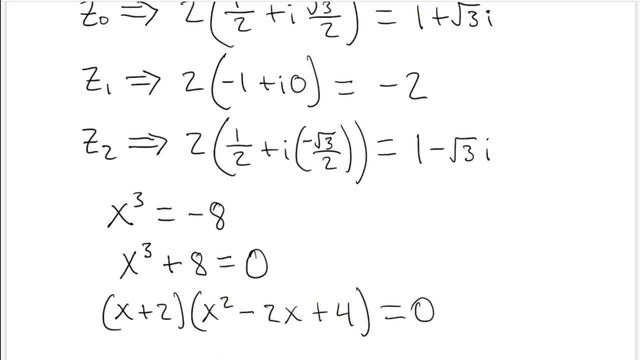 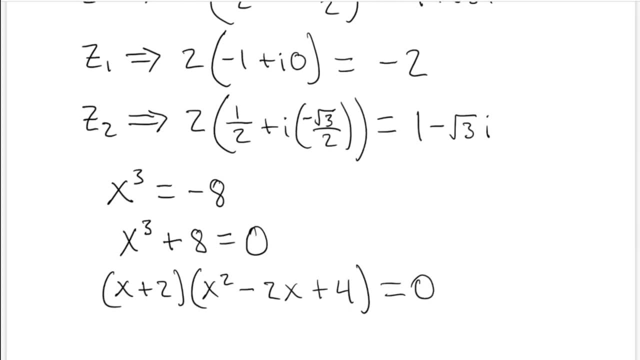 we're going to have to use the quadratic formula and we're going to get one plus or minus root 3i, so pretty cool to relate it to stuff that we've already kind of learned about from algebra. but that's all i really have for this video. hopefully you found it helpful. this stuff really just takes. 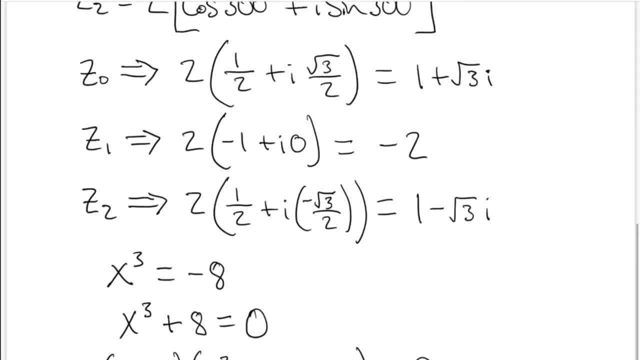 practice, you know, keep working out examples, keep thinking about this and keep flexing those brain muscles and i'll see y'all in the next video.